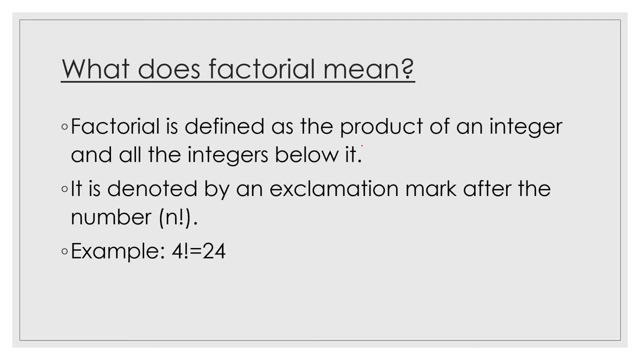 below it It is denoted by an exclamation mark after the number as n factorial. For example, 4 factorial is equal to 24, because it is defined as 4 x 3 x 2 x 3, is 4 x 3 x. 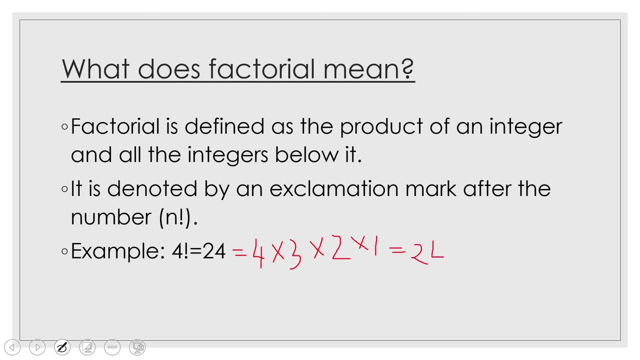 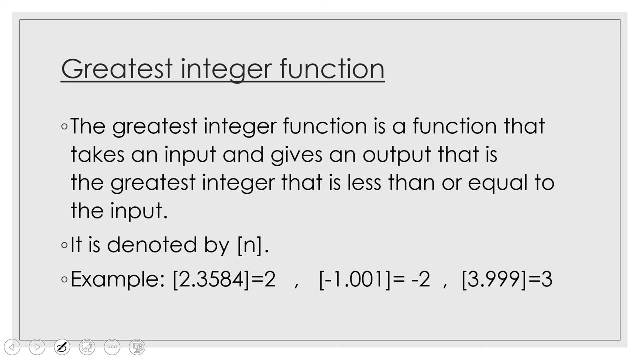 into 1, which is equal to 24.. Similarly, n factorial is equal to n, into n-1, into n-2, which continues till 1.. Greatest integer function. The greatest integer function is a function that takes an input and gives an output. that is the greatest integer. less than or equal to the input. It is denoted. 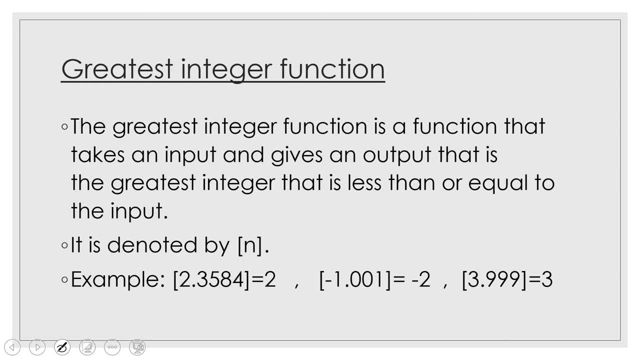 by n in square brackets. for example, 2.3584 within square brackets will give us 2, because the greatest integer less than or equal to 2.3584 is 2.. similarly – 1.001 with square brackets will give us minus 2 and 3.999 with square brackets will give us 3.. 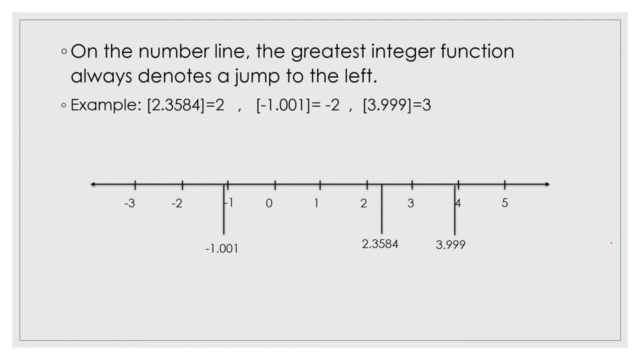 On the number line. The greatest integer function always denotes a jump to the left. For example, we can plot 2.3584 somewhere over here. So with a jump to the left we land on 2, which is the answer. We can plot minus 1.001 somewhere. 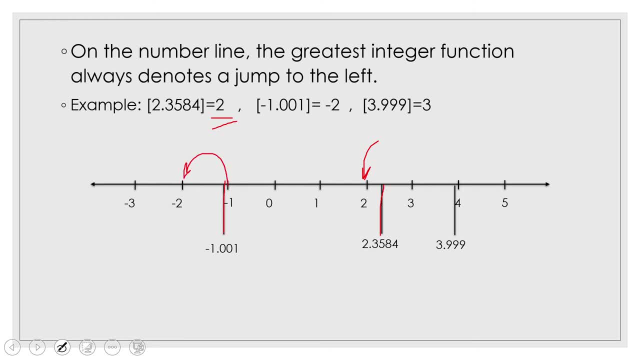 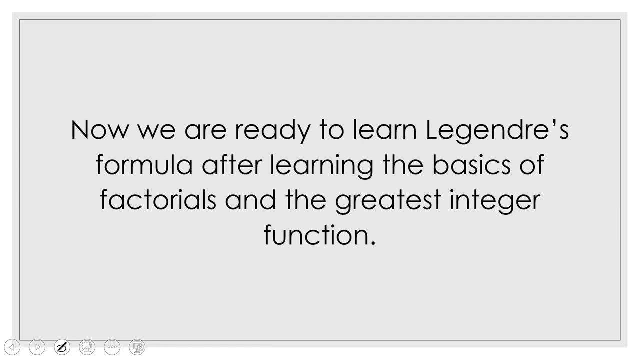 over here and a jump to the left will lead us to minus 2.. Similarly, the answer for the greatest integer function of 3.999 will be 3.. Now we are ready to learn Legendre's formula, after learning the basics of factorials and 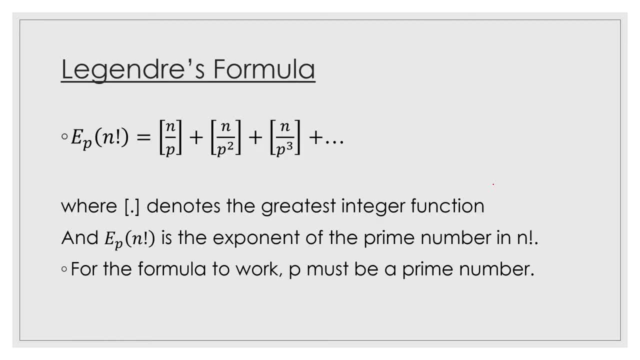 the greatest integer function. Legendre's formula. It is defined as: ep, which is the exponent of p in n factorial, is equal to square brackets n by p plus square brackets n by p, Where the square brackets denote the greatest integer function, and ep of n factorial is: 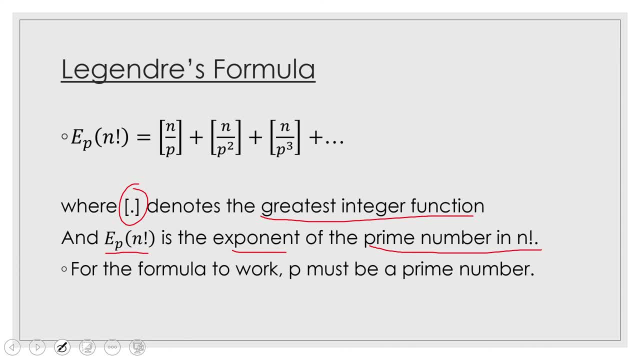 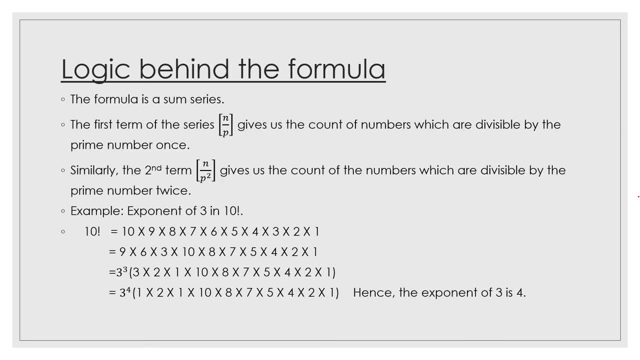 the exponent of the prime number in n factorial. For this formula, p must be a prime number. What is the logic behind the formula? The formula, the Legendre's formula, is a sum series. It is a sum of several terms, The first term of the series, which is 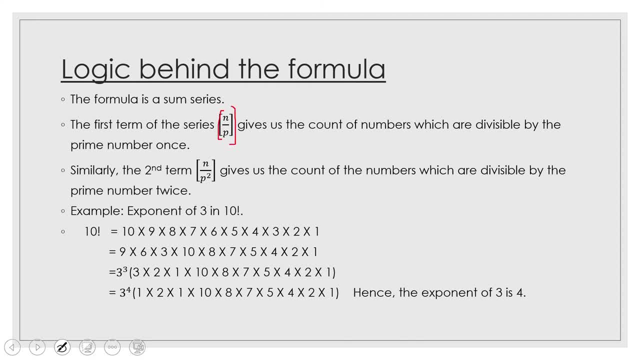 n by p within square brackets gives us the count of the increasing numbers that are divisible by the prime number once. The second term, which is n by p into square brackets, gives us the count of minus p in n factorial twice. For example, if we wish to calculate the exponent of 3 in n factorial as 10 x 9 x 8 x 7 was. 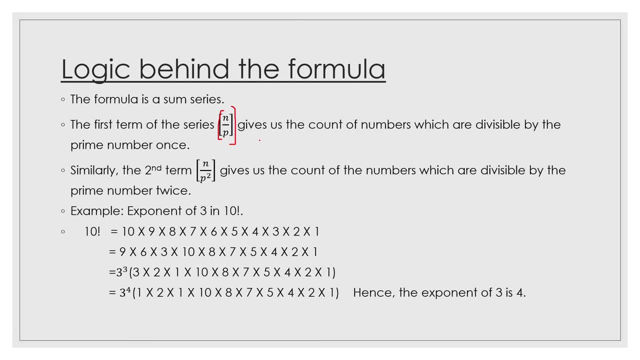 outcome in n factorial 10 x n factorial will be 10 x 9 x 8 x 7, and so the column will be thinner. Similarly, if we wish to calculate the exponent of 3 in n factorial, 10 x 9 x 8 x 7 will be: 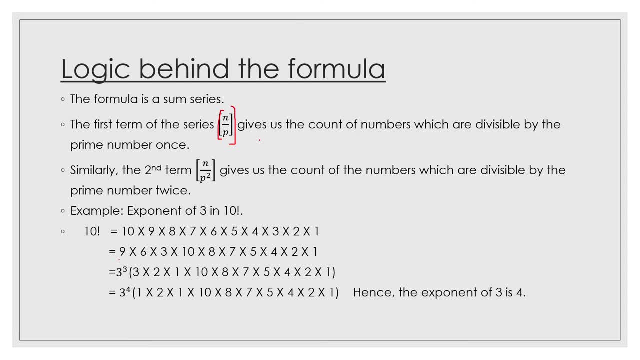 10 x 9 x 7 x 8 x 9 x 9 x 9.. Now we can take all the multiples of 3 on one side, which are 9,, 6 and 3, and write the rest on the other side. 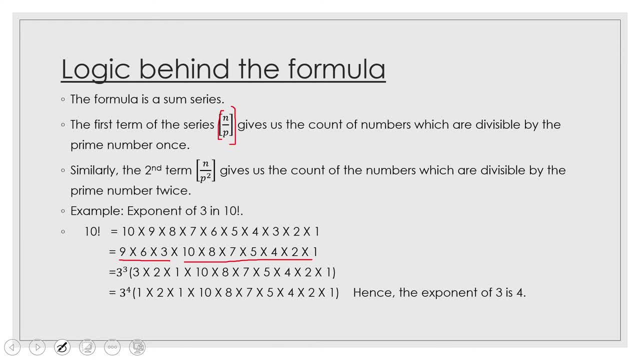 Now, if we take one 3 from each of the multiples, we get 3 cube and we can write the rest as it is. Now, if we take a 3 for the second time, we can take it only from this 3.. So now we get 3 raised to 4 and we can write the rest as it is. 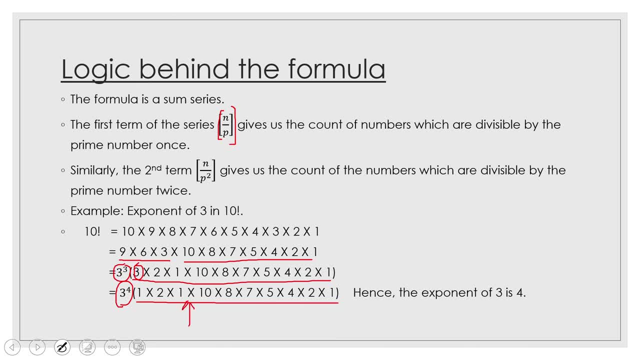 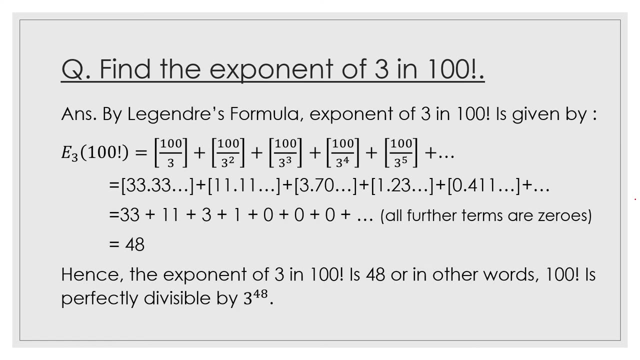 Now this part cannot be divided by 3 anymore, So the exponent of 3 in 10 factorial is 4.. Now we shall deal with some examples of the formula. The question is: find the exponent of 3 in 100 factorial. 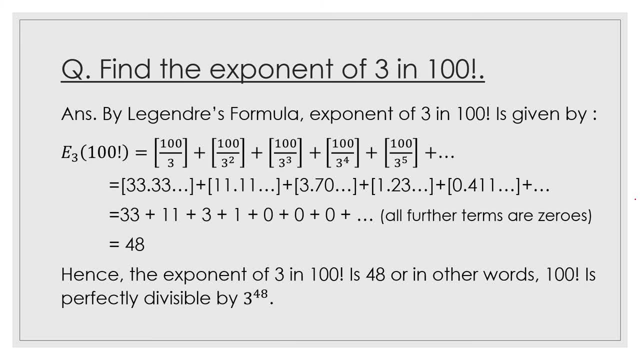 By Legendre's formula. the exponent of 3 in 100 factorial is given by. It is given by this expression. Now, if we simplify 100 by 3,, 100 by 9,, 100 by 27,, 100 by 81 and so on, we get this result. 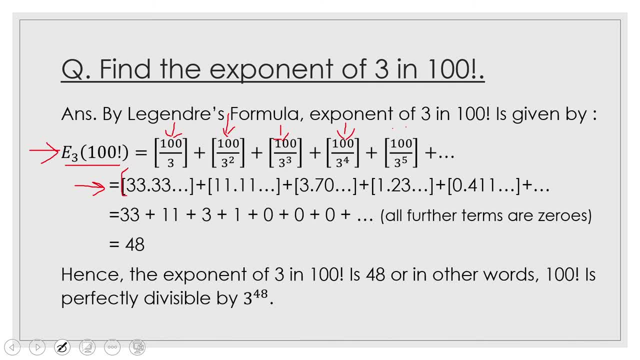 Now, if we solve the greatest integer functions, which are denoted by the square brackets, we will get these values, which are 33,, 11,, 3, 1 and the next few, not few. all the next terms will be 0.. 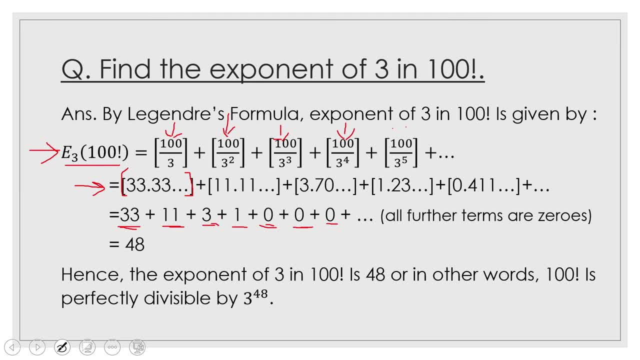 Now, if we sum up all the non-zero terms which over here are 33,, 11,, 3 and 1,, we will get the result as 48, which is our answer. Hence, the exponent of 3 in 100 factorial is 48..